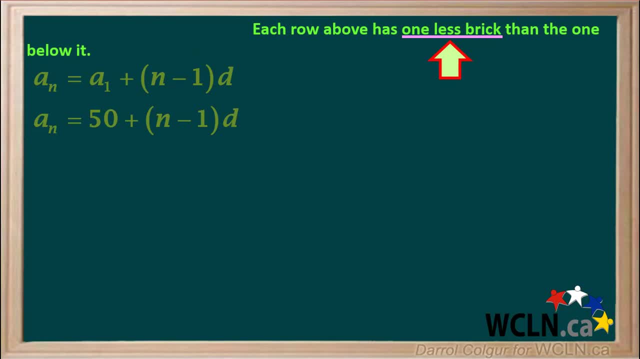 each row above has one less brick than the row below it. So each time we go up one row, the number of bricks decreases by one. This means we can give the common difference d a value of negative 1.. Now we have the equation: a- n equals 50 plus n, minus 1 times negative 1. The wall is 15. 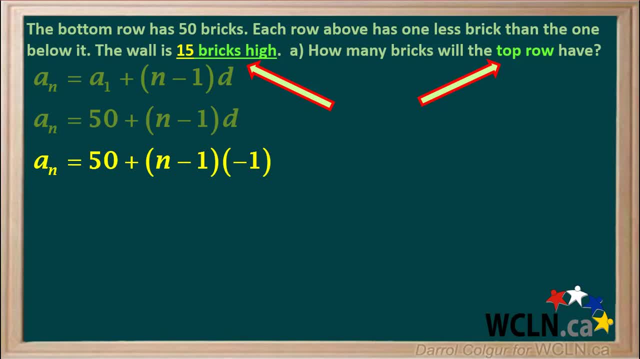 bricks high, so it has 15 rows. We are asked how many bricks there are in the top row, which is the 15th row. Therefore we can say that n equals 15.. So a n is a 15 and n minus 1 is 15 minus 1.. 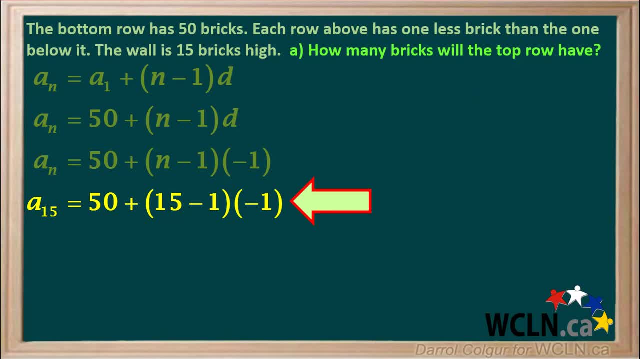 Now our equation is: a 15 equals 50 plus 15 minus 1, times negative 1.. And the value for a 15 will tell us the number of bricks there are in the 15th or top row. 15 minus 1 equals 14.. So we will. 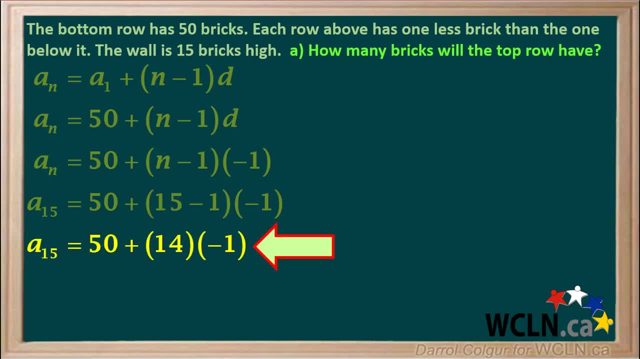 write 14 in here, Giving us a 15 equals 50 plus 14 times negative 1.. 14 times negative 1 is negative 14.. So we have a 15 equals 50 plus negative 14. Which is the same as 50 minus 14.. 50 minus 14 equals. 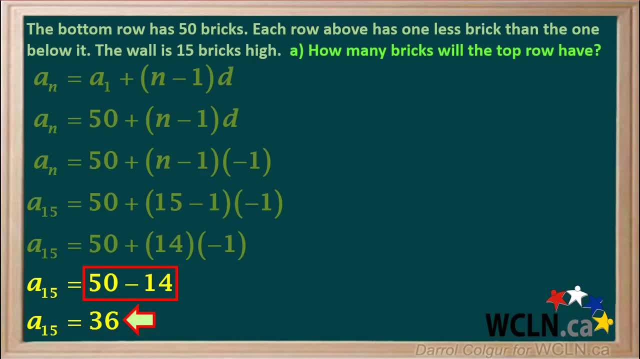 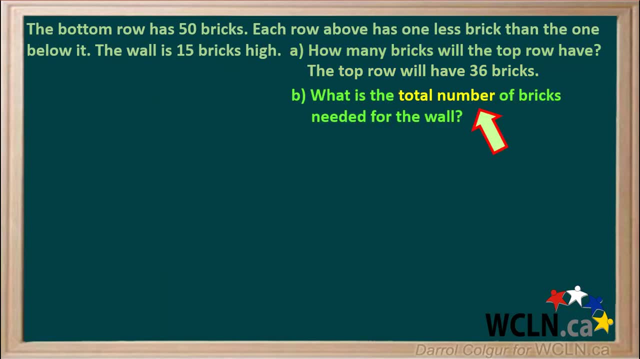 36.. So we can say that the value for a 15 is 36.. Which means the top row will have 36 bricks. The b part of this question asks for the total number of bricks needed for the wall, Knowing that term, a 1. 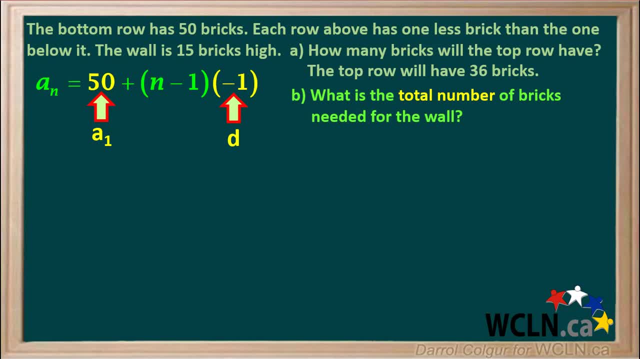 is equal to 50 and d equals negative 1.. We can write the sequence with all the terms a 1 to a 15. It starts at 50 for the number of bricks in the bottom row and ends in 36 for the number of. 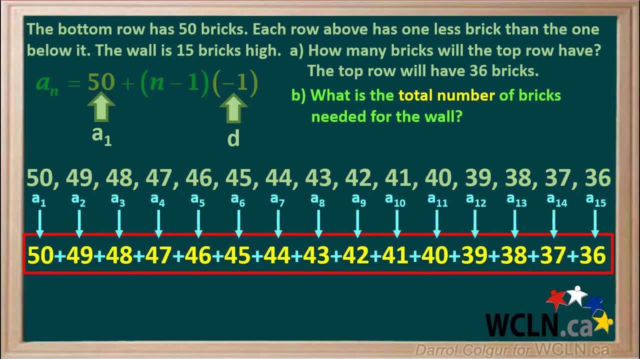 bricks in the top row. The total number of bricks will be the sum of all the bricks in all the rows, So it will be the sum of all of these numbers. Adding up all these numbers gives us a grand total of 600.. So now we know that we need 645 bricks for the whole wall. 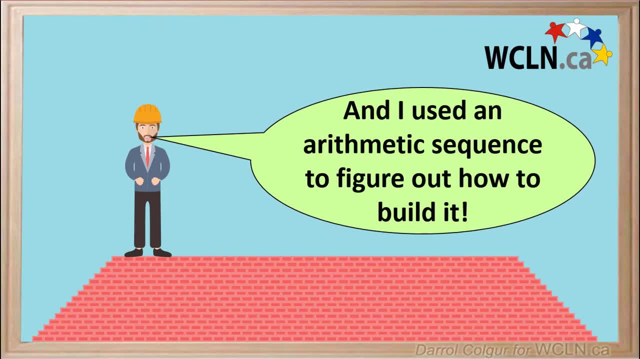 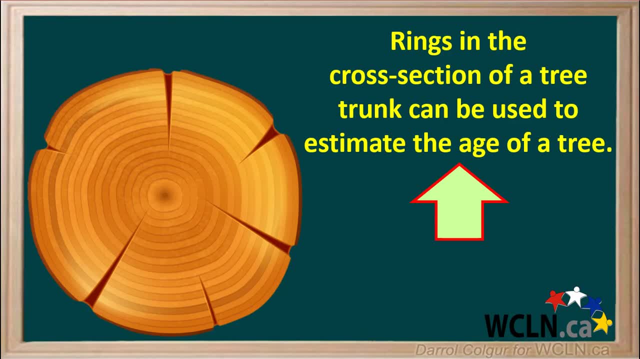 Let's look at another example of a word problem. Rings in the cross section of a tree trunk can be used to estimate the age of a tree. Each ring corresponds to one year of growth. The core of a tree was drilled out of its trunk. The core showed all of the annual 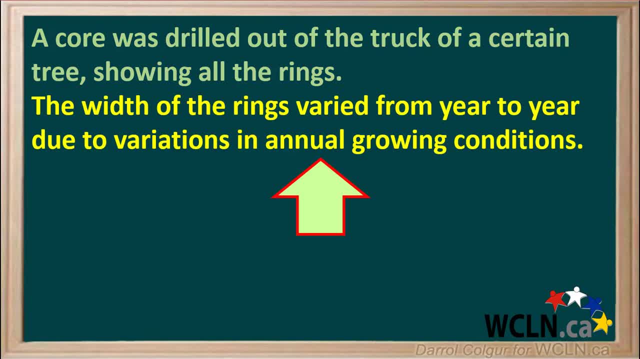 rings of growth. That's why it was named a ring The length of a tree, 3 times. The width of the rings vary a bit from year to year due to variations in annual growing conditions. However, an average of the width was taken and found to be 9mm. 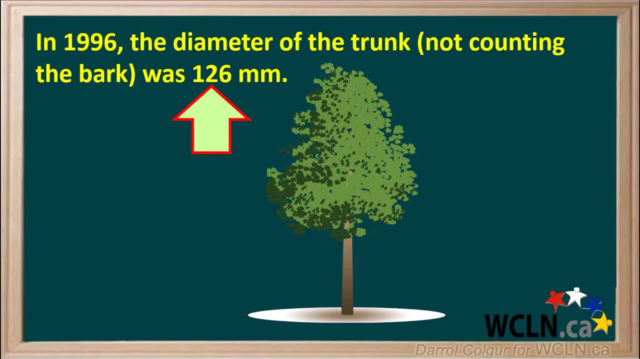 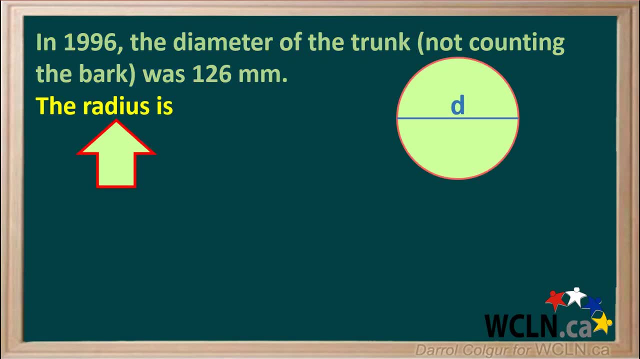 In 1996, the diameter of the tree, not counting the bark, was measured and found to be 126mm. The radius of a circle is ½ the diameter. Once again, this is because the diameter of a ring was an octalom DVD and not the diameter of the trunk. 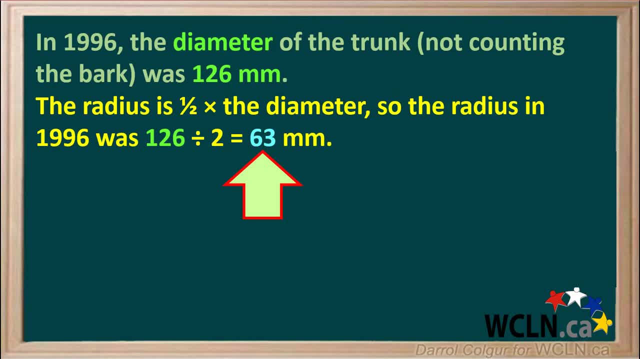 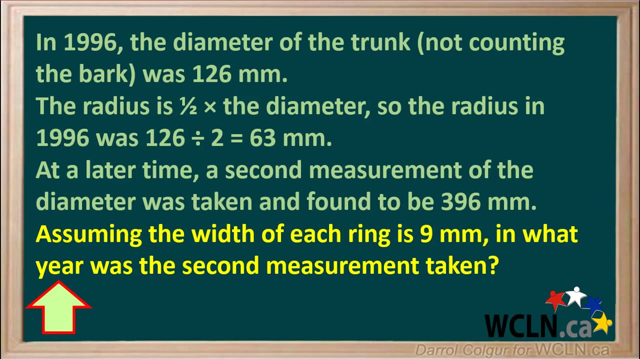 trunk in 1996 was 126 divided by 2, or 63 millimeters. At a later time, a second measurement of the diameter was taken and found to be 396 millimeters. Assuming the width of each ring is 9 millimeters, we are asked to find the year in which this 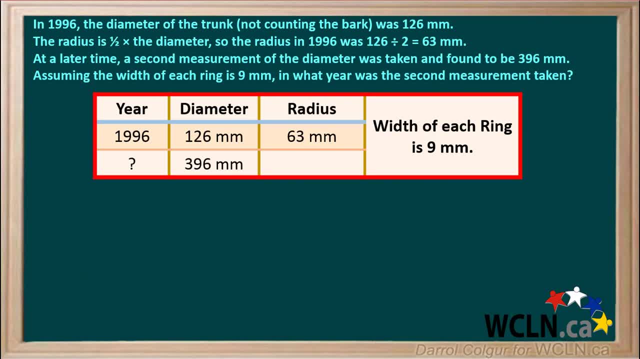 second measurement is taken. We can summarize all the information given in a table like this: The radius of the trunk in the second measurement was half the diameter, or half of 396 millimeters, which is 198 millimeters. We'll use an arithmetic sequence to help us answer this question. 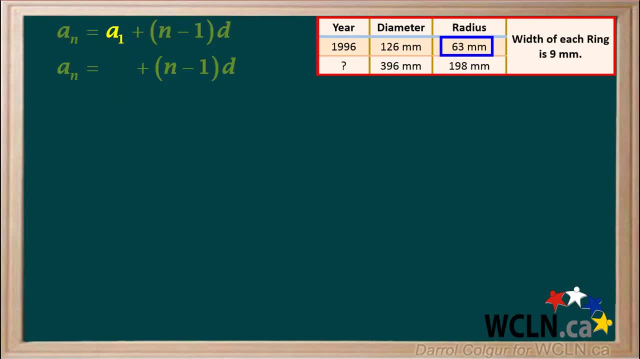 Here is the general formula for an arithmetic sequence. The radius in the first measurement was 63 millimeters, so we'll say the value for the first term, A1, is equal to 63.. The radius in the second measurement was 63 millimeters, so we'll say the value for the 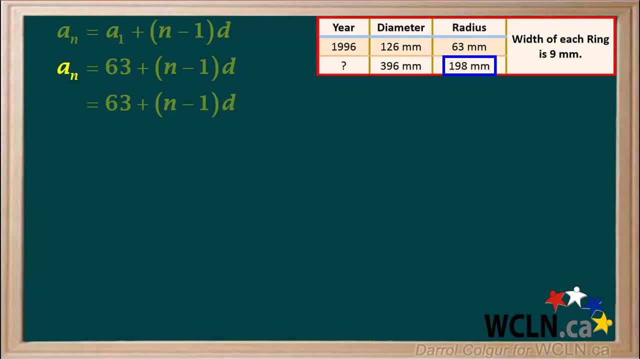 second measurement is half the diameter, or 198 millimeters. We'll set this as the value for term AN. The width of a ring corresponds to the annual increase in the radius. so each year the radius increases by 9 millimeters. Therefore we can say the common difference D is equal to 9.. 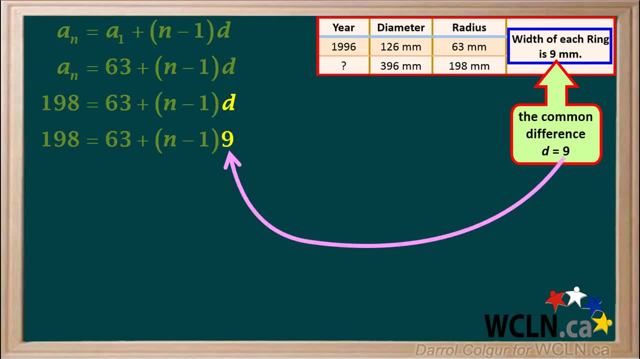 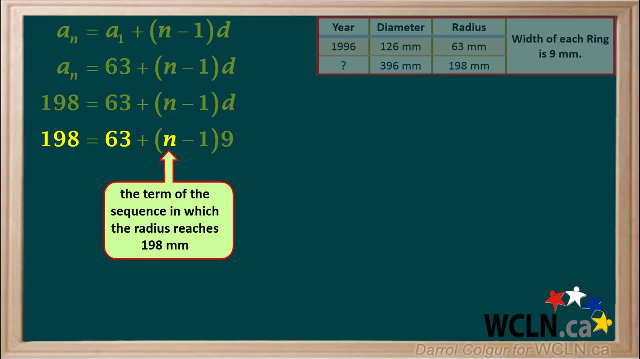 And we can put 9 in for D in this equation. Now we have the equation 198.. 198 equals 63 plus n minus 1 times 9.. Solving for n will give us the term of the sequence in which the radius reaches 198 millimeters. 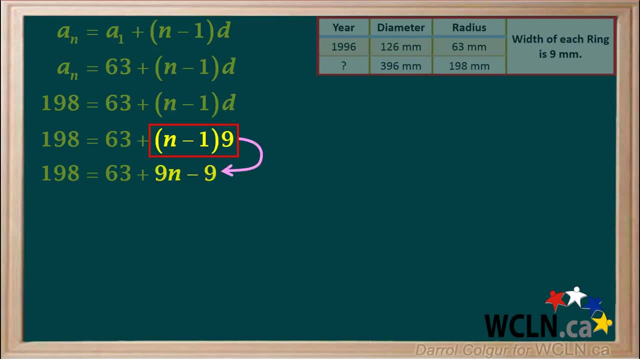 n minus 1. in brackets times 9 is equal to 9n minus 9.. 63 minus 9 is equal to 54. So we now have the equation 198 equals 54 plus 9n. Rearranging this to put the 9n on the left side gives us 9n equals 198 minus 54.. 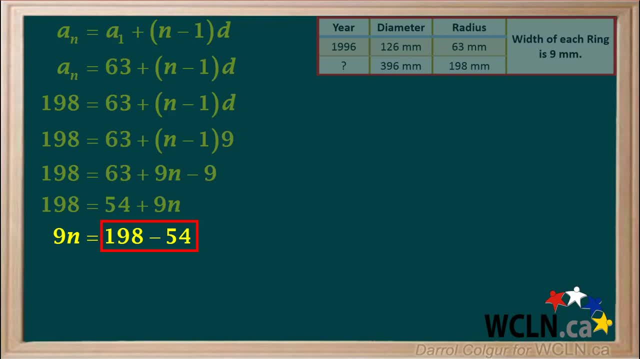 198 minus 54 equals 144.. So we can say that 9n equals 144.. To solve for n, we divide both sides by 9, giving us n equals 144 divided by 9, which works out to 16.. 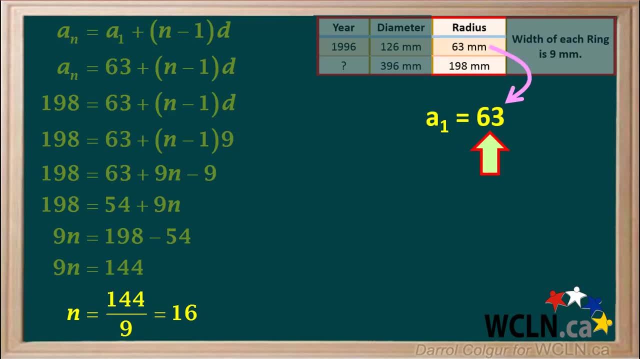 So we now have the equation 198 minus 54 plus 9n. We know that term A1 is equal to 63.. And term AM, which we now know is term A16, is equal to 198.. The first measurement A1 was taken in 1996.. 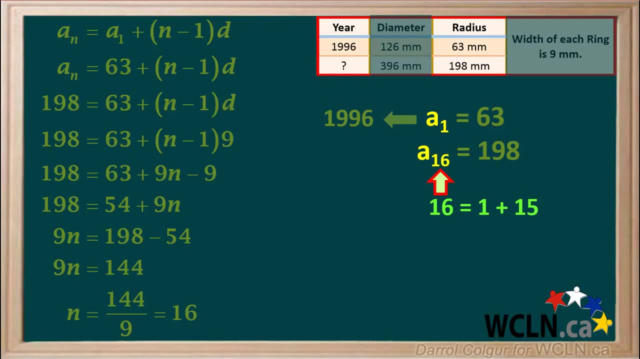 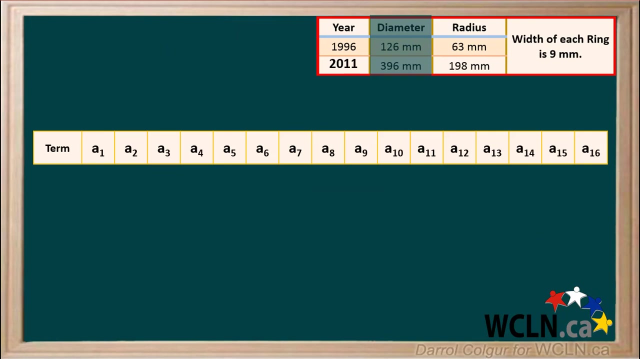 16 equals 1 plus 15,, which means 15 years after 1996 is 1996 plus 15.. Which is 2011.. So we can state the second measurement was taken in the year 2011.. To check this, we'll make a table with all the terms A1 to A16.. 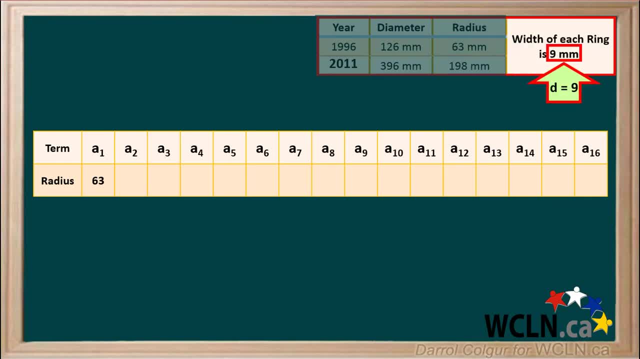 The value of term A1,, which is the first radius measured, is 63 millimeters. The width of each ring is 9 millimeters, so the common difference d is equal to 9.. This means the radius should increase by 9, and we can then take the radius of each ring. 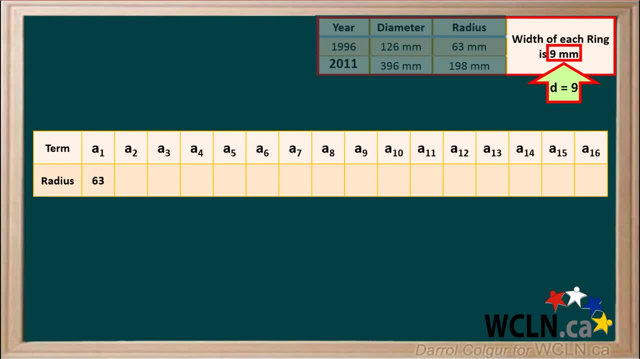 by 9,, which is equal to 8.. by 9 for each consecutive term. So the second term, A2, is 9 more than the first term, A1, or 63 plus 9,, which equals 72..